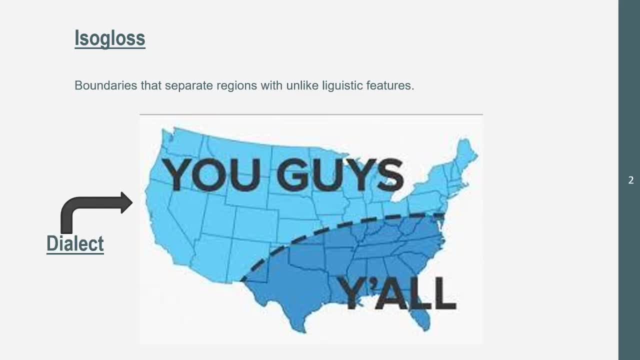 actually a dialect too. A dialect is where there's one language. However, depending on where you are, that language will have different pronunciations or a different way it is written. So this map is an isogloss and it's also a dialect, Because the isogloss it shows the 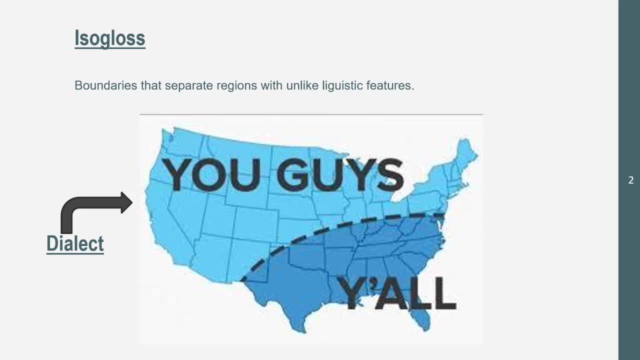 boundary of where they say you guys and y'all. However, the dialect is saying you guys or y'all. It's basically just pointing out to multiple people. Now, a dialect can also be written. So in Britain, in the United States, you still say theater, of course with the different accents. 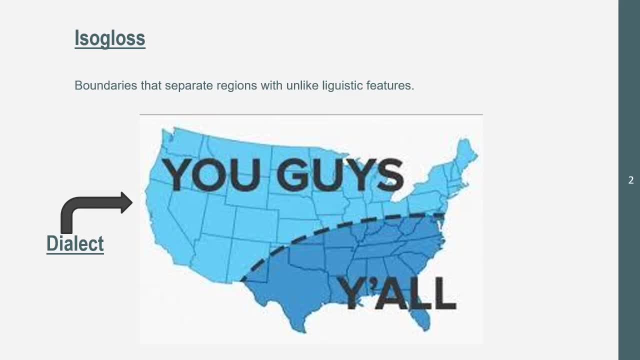 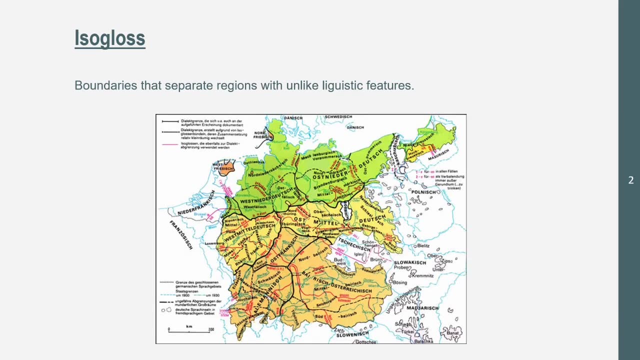 but it's still theater. However, it is written differently. That is also a dialect, and you can also show that in isogloss. Now, an isogloss can be this advanced as well. It doesn't have to be this simple. It can be this advanced as well. Now let's get into language families, which is a group. 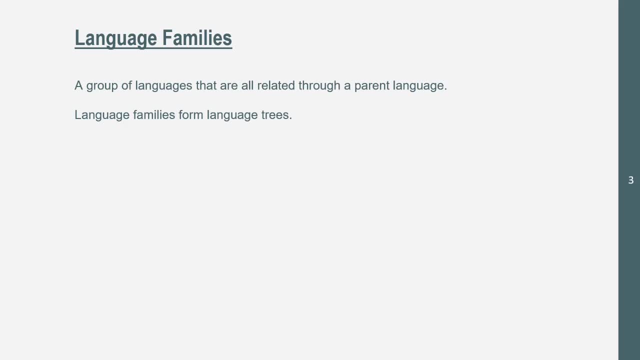 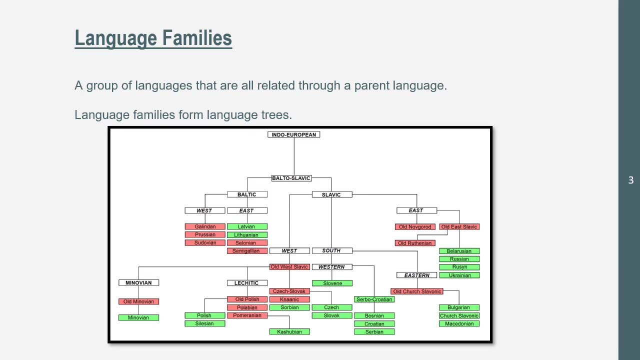 of languages that are all related through a parent language Language. families form a language tree, and a language tree can look like this: something you put in your biology or genetics class when you're making a family tree. However, it's for languages. 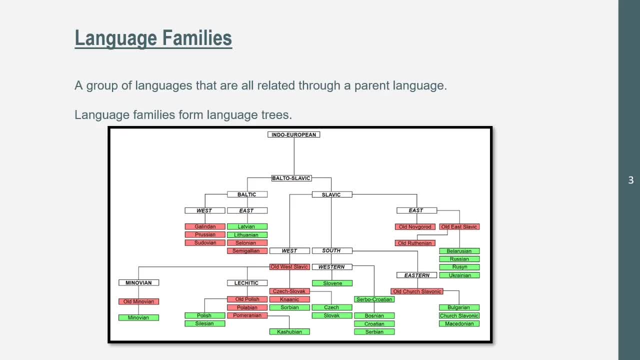 This language family is actually Indo-European. and then we have our language branches. We have our Slavic- I don't know if I'm pronouncing that right. You can't see the Romance languages on here. We also have Eastern, We have East Baltic or Baltic. I don't know how to pronounce those. 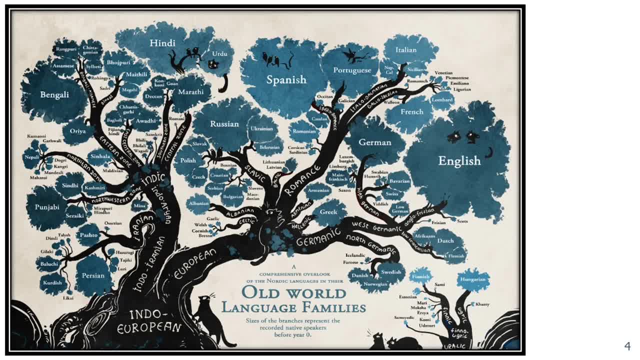 but this is a language family. A language family can also form an actual tree like this, and then the trunk of the tree is going to be your language family. Now your language branches. Of course it can be your branches. So we have. 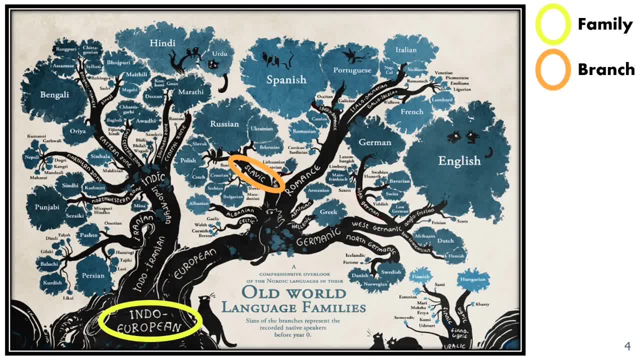 our Slavic languages, We also have Germanic languages. We also have Romance languages. You can see them now. I think you can see my mouse. So there's our Romance languages. Then we have our language. It's going to be the group of leaves. We have Russian circle, but there's also 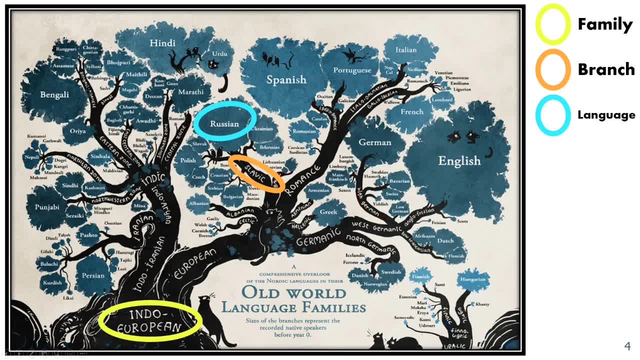 Spanish, Portuguese, Italian, English, German, French, all the other Indo-European languages on here. And then I like to say that the leaves are our dialects or our words that make up the language. You can disagree with me if you like. That's not something you need to know. 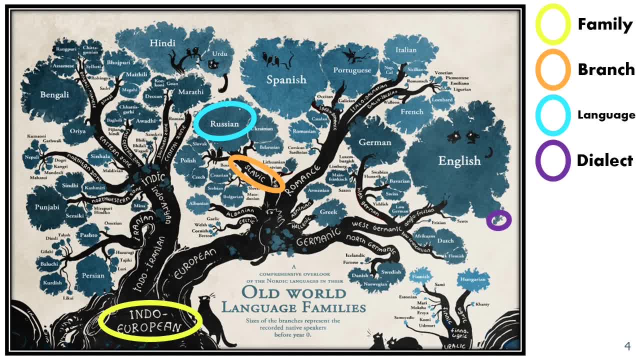 but I do like to point out that I think the leaves are kind of your words or your dialects inside the language. So the dialects make up the language and the language makes up the branch and the branches makes up the family And of course we have our leaves mix up the branches. 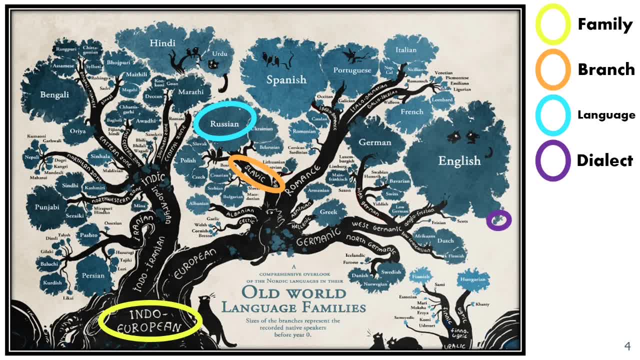 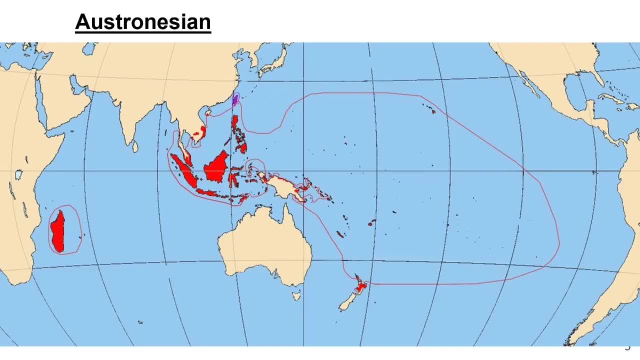 and then our branches mix up the tree, So it's like the same thing. That's why we have language family trees. It's just easy to do. All right, let's get into some language families. I think there's like six or seven we're going to go over. 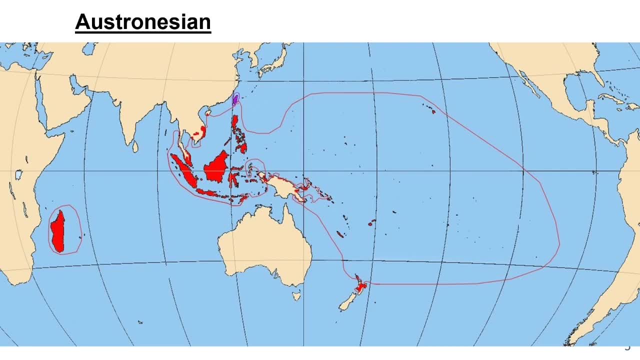 We already went through one which is Indo-European, So we have our languages like English, French, German, Portuguese, Hindi. So that's the Indo-European language. Here we got Austronesian language family. You can kind of see where this is based. I didn't look up any. 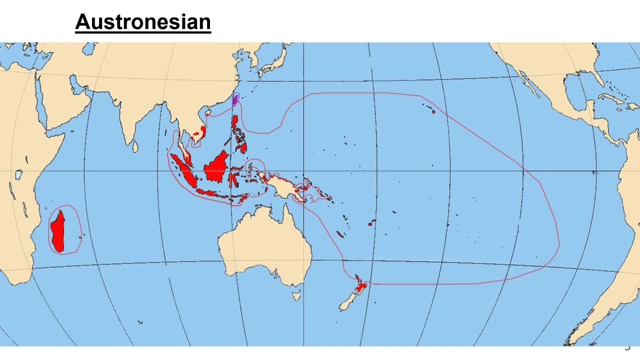 languages in this language family. So if you know any, that's great. But as you can see here, it's primarily based in Indonesia, basically Southeast Asia, and then Madagascar, which is a part of Africa, So we have you know. Madagascar, which is a part of Africa, So we have you know. 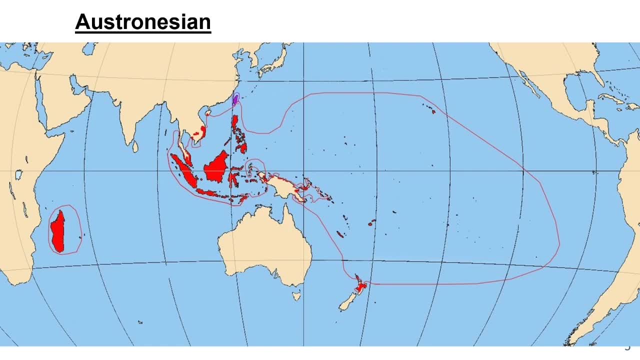 Madagascar, which is a part of Africa. So we have, you know, Madagascar, which is a part of Africa. We have Southeast Asia, Asia, we have a little bit of Northern New Zealand as well. We have Malaysia, Taiwan, Philippines, Indonesia. Those are our main countries here. Now, the hearth A. 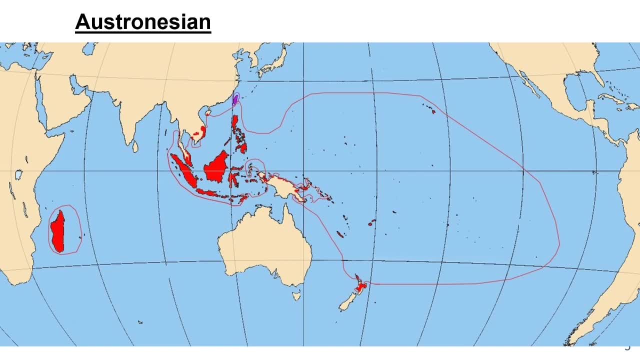 language will diffuse from a hearth, which is kind of where a language, family or religion- we'll get at it in just a second- will form and begin. So here I made the hearth. I chose this because the hearth was a different color, So figure out where the hearth was or is right. 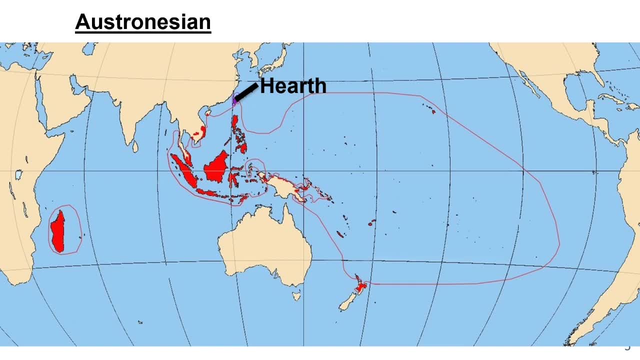 So it's going to be here in Taiwan, This is going to be the hearth, And then it diffused. You can kind of tell it kind of diffused from relocation diffusion. They migrated to other parts of Southeast Asia and Madagascar and that's how the language family has spread Most of the 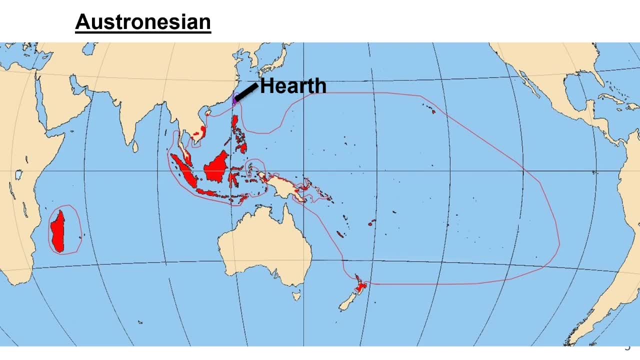 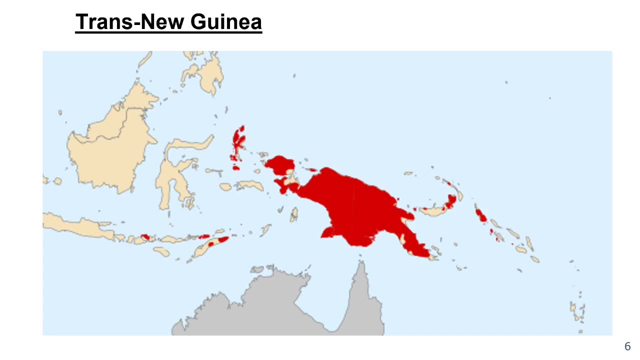 time. this is going to be through relocation, diffusion of language families. A religion will be through relocation and contagious diffusion. We'll get in that in a little bit Trans-New Guinea. This is basically the Southeast Asia that is not Austronesian, It's Trans-New Guinea And it's just kind of the other parts of Indonesia, right. 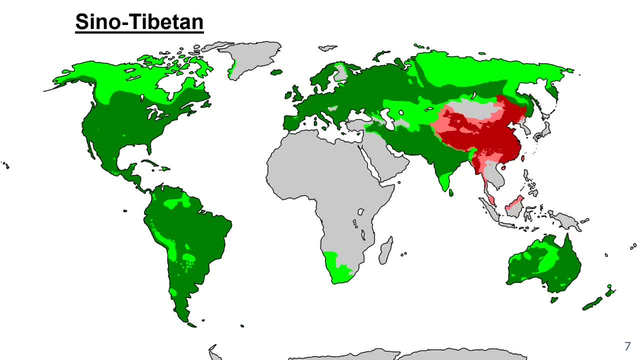 there And you can tell where the hearth is for that Pretty, pretty simple Sino-Tibetan. All right, So the red is where the language is spoken the most, And then the green is where it is spoken. 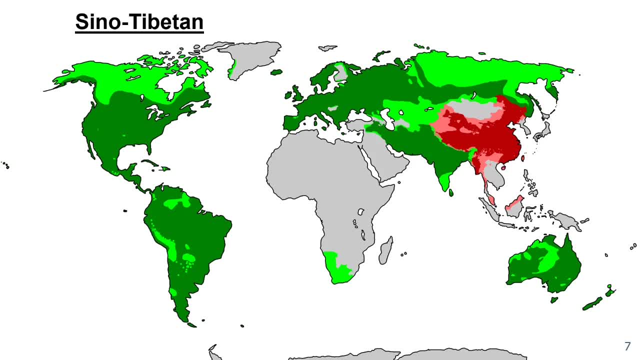 the least. So the lime is spoken the least And you can probably tell, okay, a language that's already part of Sino-Tibetan, which is Mandarin, And Mandarin's hearth is in China. This is kind of in Northern China. It's the Sino-Tibetan. 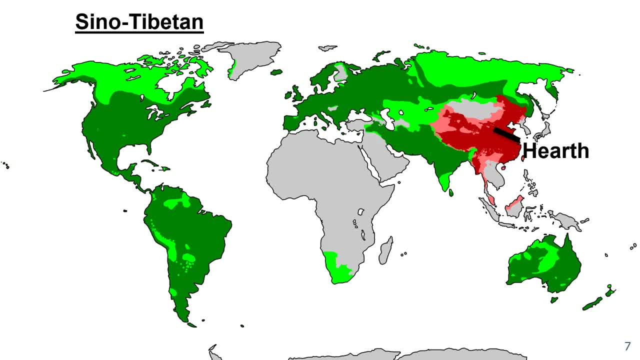 Now you can also tell- okay, but it's sorry. spoken around the world. Well, Mandarin, as you know, is the most popular language in the world, And then people have communication with China. Some people use Mandarin as a lingua franca. I believe that's how you pronounce that too. So it's no. 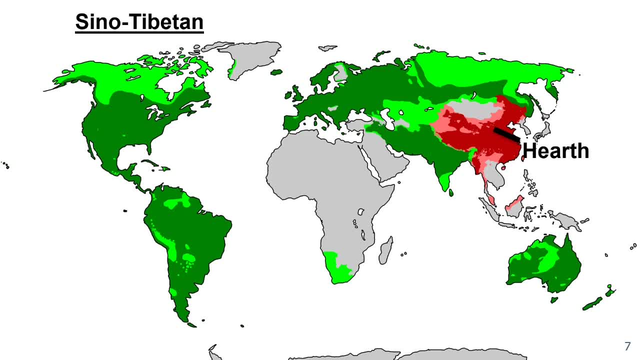 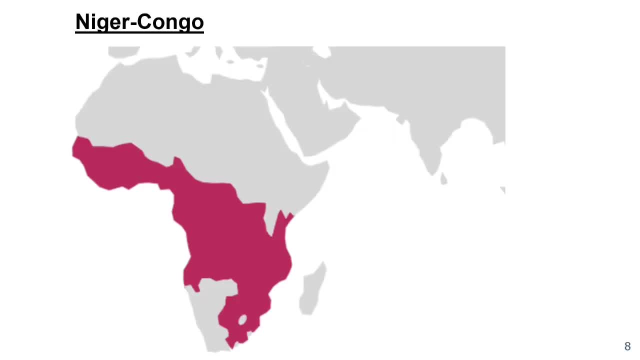 surprise that it is spoken around the world. And, of course, China is very densely populated, So there's going to be some very dark red on this map, But that is Sino-Tibetan Niger-Congo, even though Niger is not highlighted. pink. 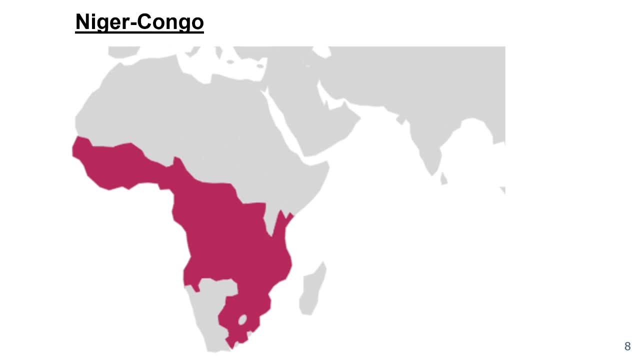 Or violet or however you want to say, your color. This may look yellow for colorblind people, I don't know. However, Niger-Congo: we kind of got a lot of middle in a little bit of Southern Africa. We got like Tanzania in here or Nigeria, as highlighted there. Niger-Congo languages, if you know any. 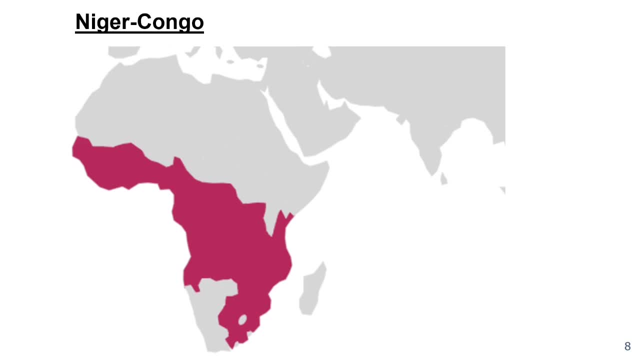 languages in Africa. I can't think of any off the top of my head either. That's where they're going to be. Kind of see where this is highlighted and kind of get an idea. You're not getting that Western part of Africa, nor you're getting the Northern parts as well. Now the opposite of Niger-Congo. 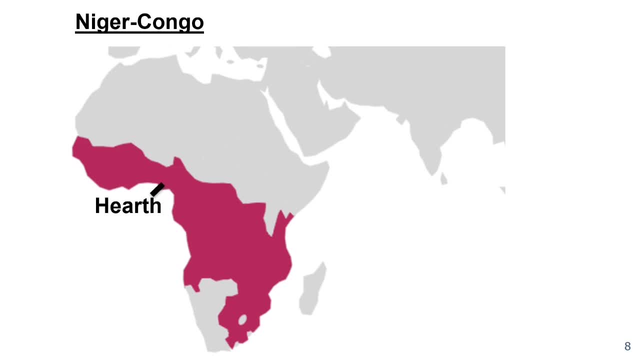 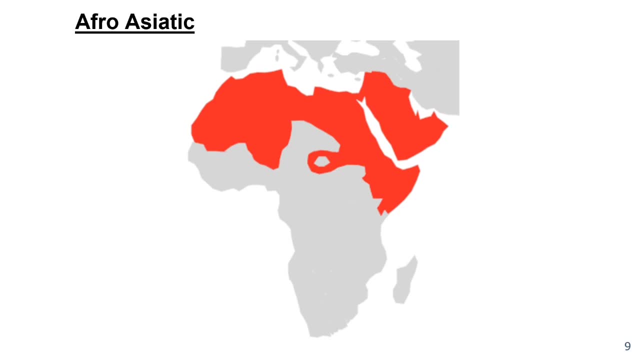 I like to say sorry. the hearth is Western Africa. Now, the opposite of Niger-Congo is your Afro-Asiatic. We have Africa and then we have Asia, and they are part of this one language family. So that's why. 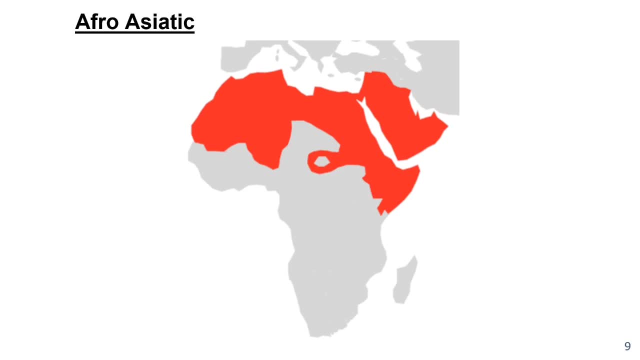 it's called Afro-Asiatic. Basically, this is Northern Africa and then a little bit of Asia, the Middle East. We have Saudi Arabia, Yemen, and we're in Africa. We have Morocco, Egypt, Algeria as well, and those are your Afro-Asiatic languages. There's those Middle Eastern. 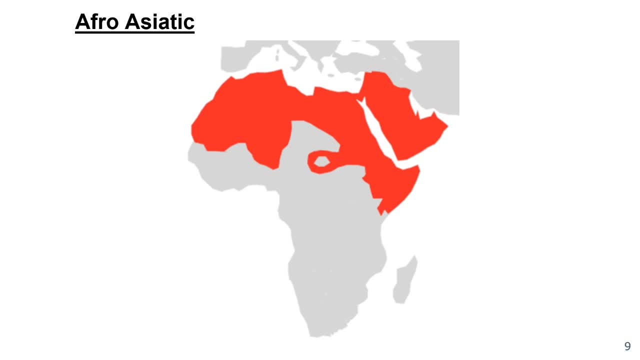 languages. Arabic might be part of Afro-Asiatic. It might not be as well. I believe it is. Don't take my word on that, though. Now we'll see a similarity of the diffusion of the Muslim religion, Islam. We'll see a similarity in diffusion to this. We'll see it go over Northern Africa and 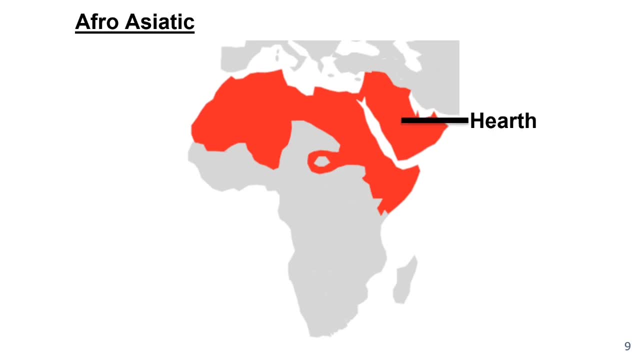 then around the Middle East And in the hearth Afro-Asiatic is in Saudi Arabia And then it diffused through relocation diffusion to Africa. because you can see it's close together, They could just migrate over there, All right. What was the choice? question: practice: Which of the following countries? 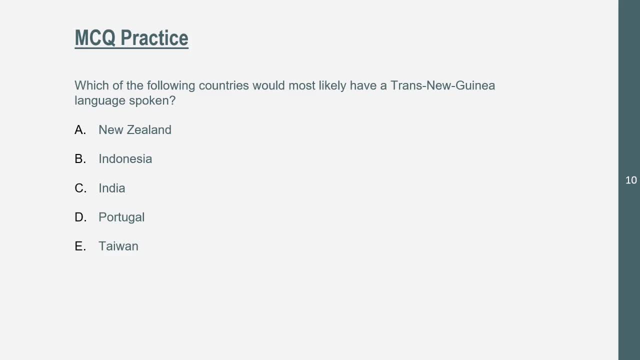 would most likely have a Trans-New Guinea language spoken. The correct answer is B- Indonesia. New Zealand would have either Austronesian or Indo-European, Not Trans-New Guinea. If you remember looking at the map, we didn't see New Zealand on there. Indonesia was on. 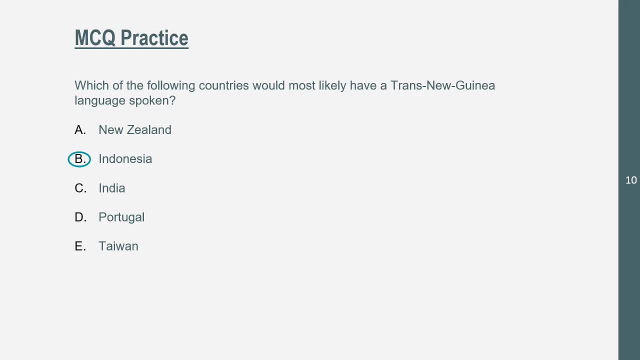 there, India wasn't. India has primarily Hindi, which is Indo-European. Portugal has Portuguese, and that's also Indo-European, And then Taiwan is Austronesian, Yeah, Austronesian, And so that leaves Indonesia. Indonesia is Austronesian, It's primarily Austronesian. actually, However, it's the only. 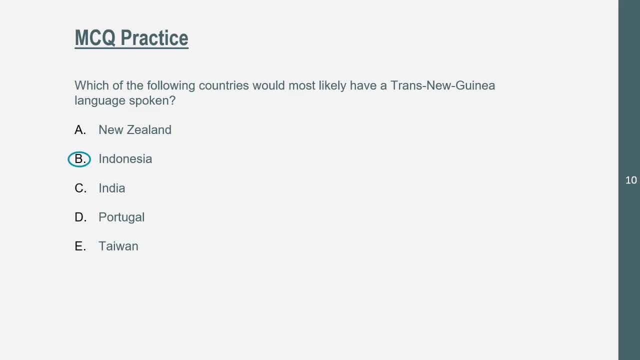 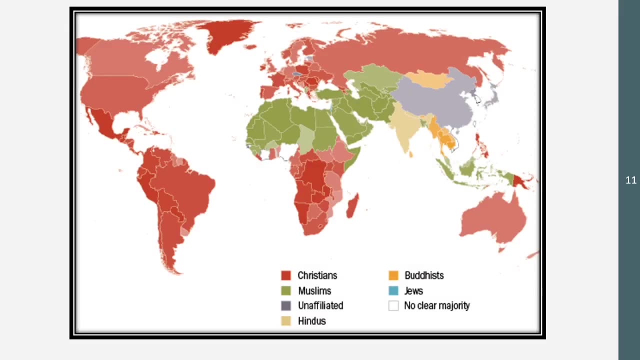 country here on our multiple choice question practice that has Trans-New Guinea languages primarily spoken. All right, Let's get into religion. So we learned with languages that they'll diffuse from their hearths And I guess it would depend how it would diffuse. A lot of times it was through. 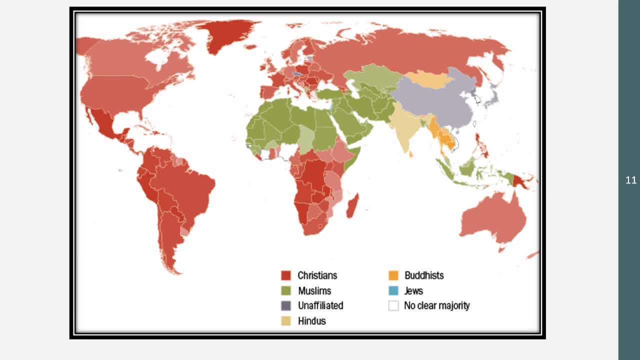 relocation diffusion. However, I want to point out that Indo-European. why did that diffuse around the world? How did that diffuse to Northern and Southern America? Not like the country, the continents, probably just the North and South America, But how did it diffuse? 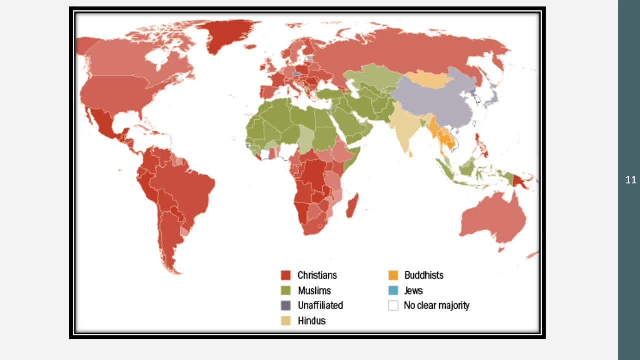 there It got to Australia. Well, things caused diffusion. You probably have learned this already- but there was imperialism and colonization through many European countries. of course, Spain, France and especially the United Kingdom, Those languages that they speak, so French. 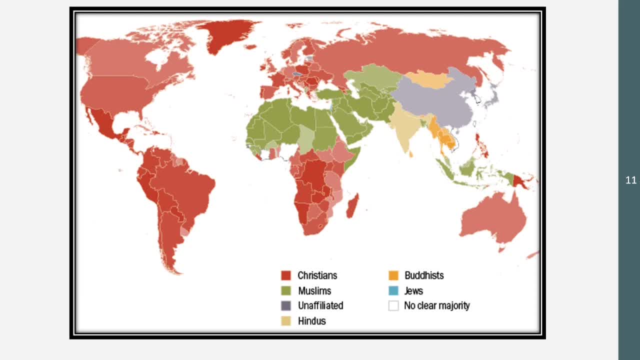 English, Spanish are primary languages of North America, South America and Australia, And that's caused by relocation, contagious diffusion and some other types of diffusion as well: Stimulus diffusion, if you think about it from some ways, words are spoken in the United. 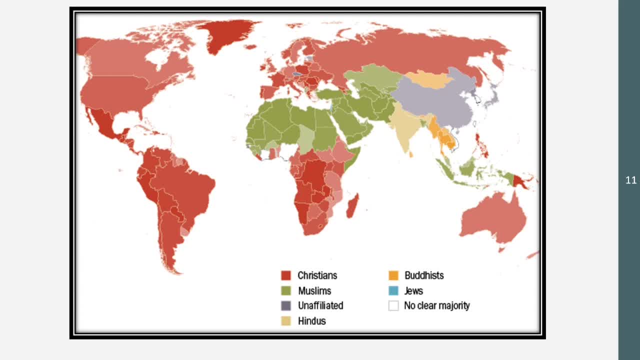 States to the United Kingdom, Britain, whatever you like to call it. Now we're tapping into religion, So you can look at this map and kind of see where the religions are primarily located. Please understand this, Please understand this map and where religions are primarily. 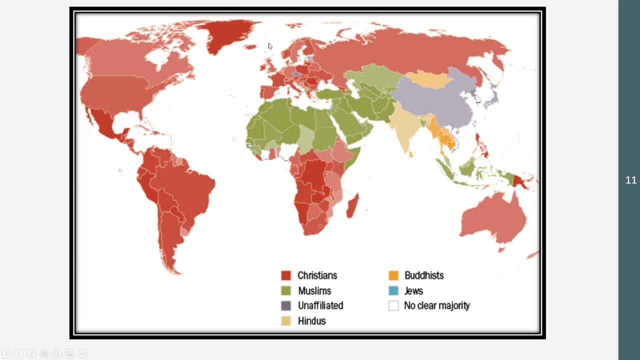 located. I do want to point out China. Even though it is unaffiliated, it has a lot of Buddhism in it. So if you see China, it's probably going to have Buddhism. If you ask for China, primarily it'll be Buddhism, Because you can see here, 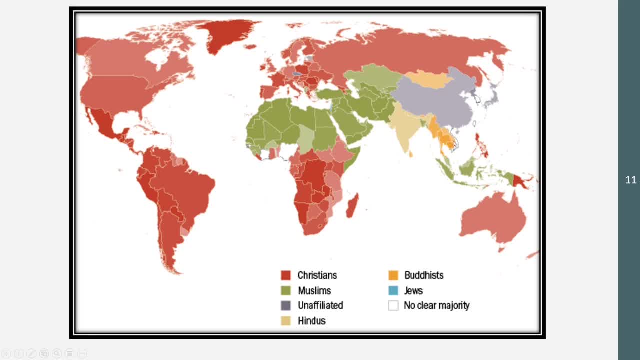 we have Thailand, Myanmar, Vietnam, Buddhism, China's right above it, It's most likely Buddhism. If you're looking for Judaism, look at Israel. Israel had a bunch of Judaism after World War II, of course, when Jewish people were escaping Germany- And then look at Islam, which is green. 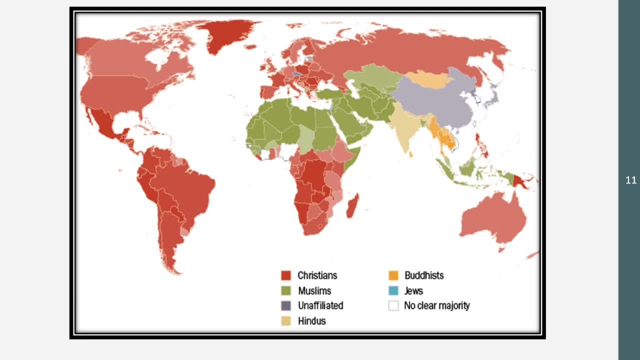 You can see that there's a similarity between Afro-Asiatic diffusion and the Islam religion. It's a bunch of Nordic Northern Africa. So when the people from the Middle East went to Africa, they probably brought the religion and the language family with them. Those are some conclusions that can be made by those two. 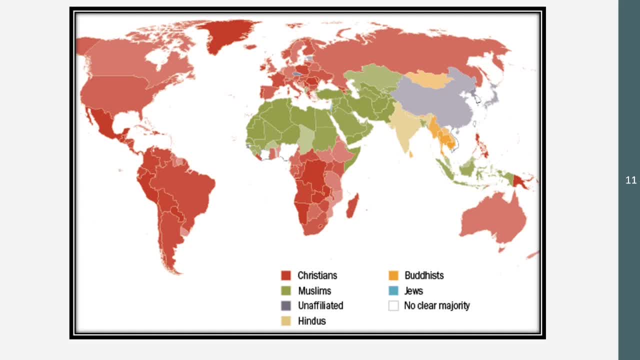 maps we've looked at. And then let's look into Christianity. Like Indo-European languages, Christianity diffused around the world: Northern, South, North and South America. I'm going to be better at that. A bunch of your, A bunch of African, I'm going to be better at that. I'm going to be better at that. 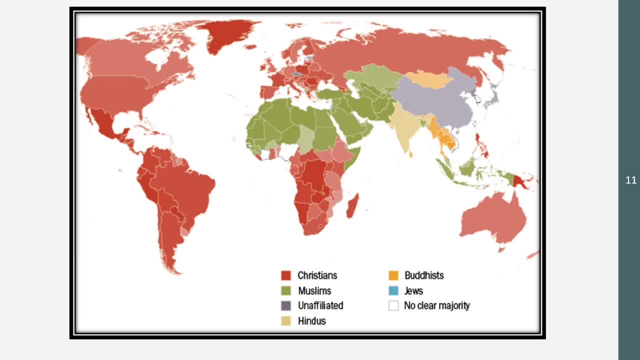 America, Australia, Russia and almost all of Europe. Christianity diffused there. Now the Christianity hearth is going to be kind of near Israel, I believe. I don't know where Christianity's hearth is. I probably should know this, though. However, why is it not there now? 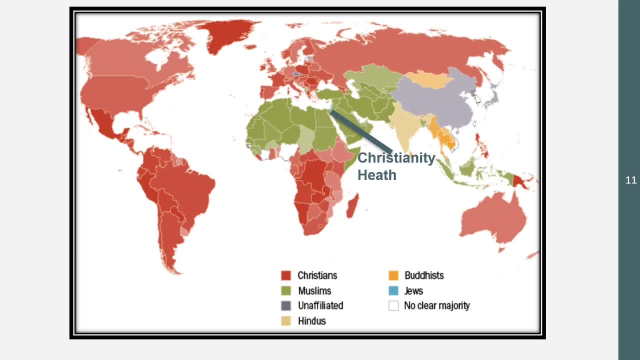 Think about that for a second. We don't see Christianity now. Like I said, Judaism took over a bunch of places in Israel and then we have Islam around that area. Christianity is older than Islam. So when Christianity diffused- if it was diffused by relocation diffusion, there's going to be less. 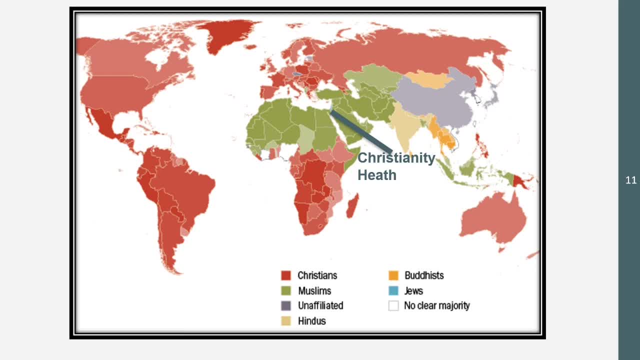 people there who are a part of Christianity, And then, when Islam blew up, it would have taken over the area and become primarily Islam. Of course, you would still have your Christianity people there. So that is something to think about Hinduism, which is part of Nepal, and 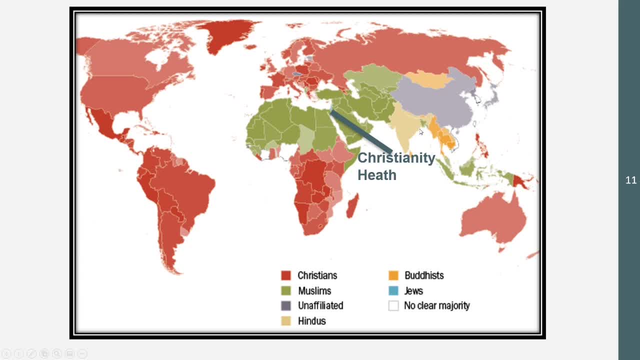 India- India mostly- is going to be one of the oldest- Sorry, one of the oldest religions. My thoughts are not coming to my mind as quick as I want them to, So it's not diffusing as well. Now, if you're thinking, 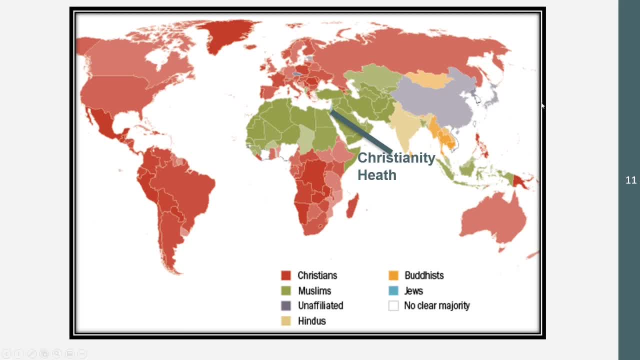 okay, it's older, Shouldn't it diffuse as well? Well, we have Buddhism around here, and we'll learn about universalizing religions and ethnic religions in just a second, And that'll explain why Hinduism is not diffusing as much as Buddhism or Christianity. 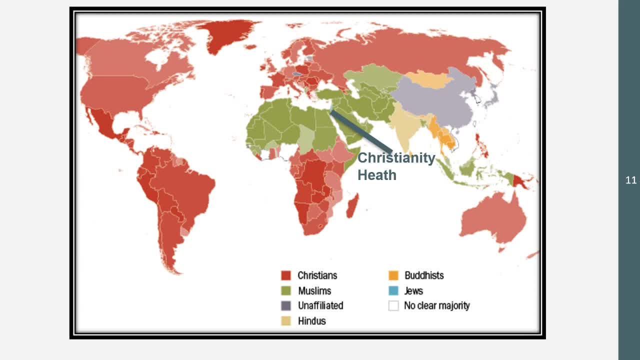 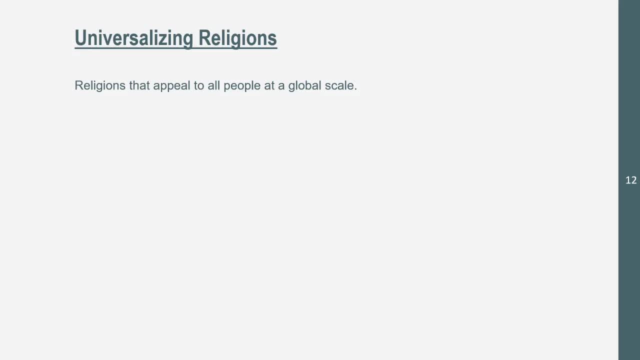 Or Islam is, And why Judaism isn't diffusing as much as a lot of these other religions are. Now universalizing religions are religions that appeal to all people at a global scale. Pay attention to what these religions are: Christianity, global scale. Christianity is literally in every. 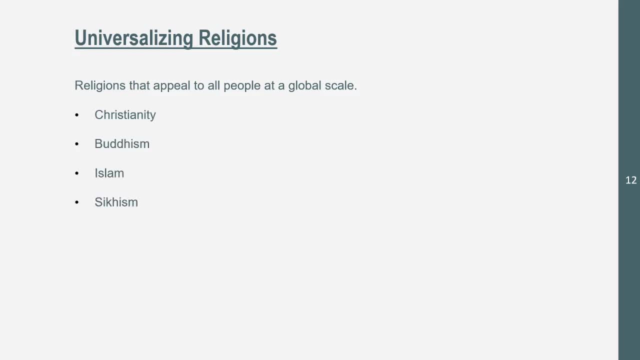 single continent. Buddhism, Islam and Sikhism. These are our four universalizing religions that you're going to have to know, And these are the four religions that take up most of the map we just saw. There's Sikhism on there, because it's not that big of a religion, It's just kind of something you 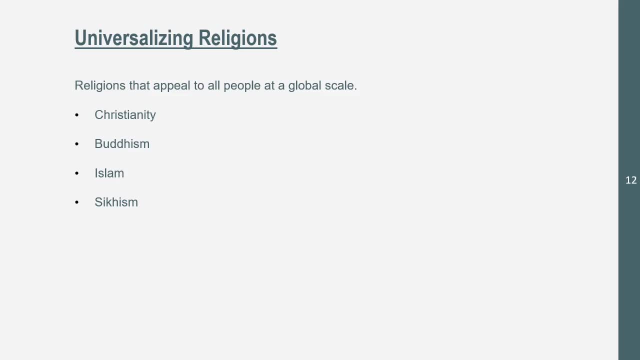 need to know as a thing. However, you don't see Hinduism and Judaism on there, because they're not universalizing, of course. However, they're also not diffusing as much. Since universalizing religions are appealing to people at a global scale, it's, of course, going to spread out more. 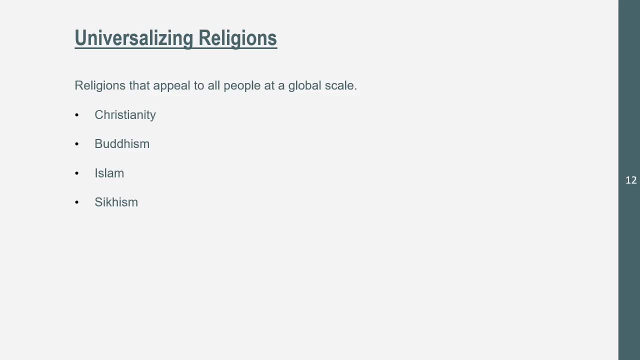 and diffuse more than ethnic religions, which is what Hinduism and Judaism are. Let's get into these four religions. We're going to learn a little bit about them. So Christianity: The hearth is in Jerusalem. I knew that when I wrote it down, but I forgot it. It was formed when a Jewish teacher named Jesus, I probably. 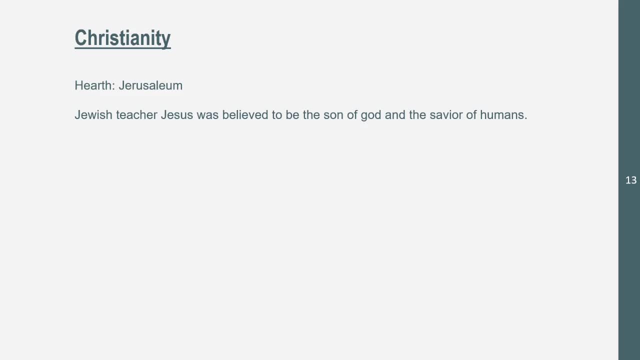 should have put a comma or something. there was believed to be the son of God and the savior of humans. The religion is monotheistic. That means they believe in one God. Their sacred text is the Holy Bible. It is spread through different types of diffusion: Contagious diffusion- An example would 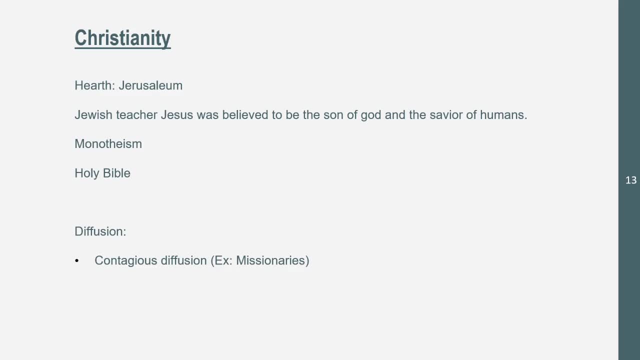 be through missionaries. So one missionary could go to someone's house preach about Christianity and then four to ten people or something could now be Christians. Hierarchical diffusion- I hope I said that right. An example would be forced upon by rulers. So maybe you live in a country and the ruler's like. 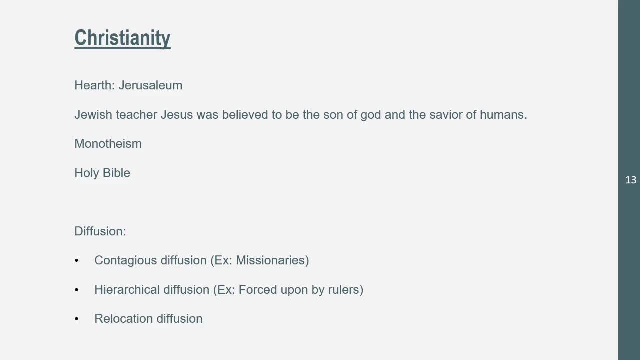 you guys have to be Christians or your heads will be cut off. And then, of course, through relocation and diffusion, which is pretty easy, Migration. All right, let's get into Buddhism. The hearth is going to be Nepal. You need to escape the cycle of suffering. So he taught around the area, and then those 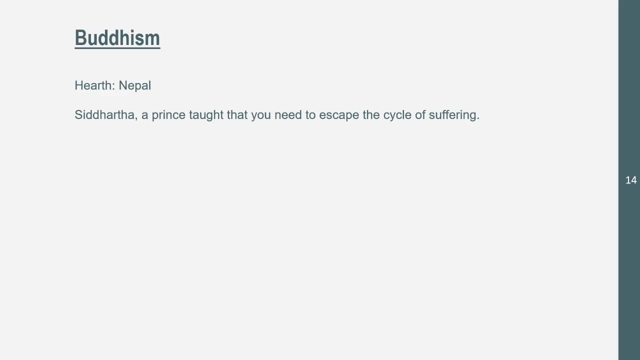 teachings didn't diffuse, especially down the Silk Road That diffused Buddhism into China. But they said you need to escape the cycle of suffering. Buddhism is neither monotheistic or polytheistic, So they don't believe in one or multiple gods, And their sacred text is: 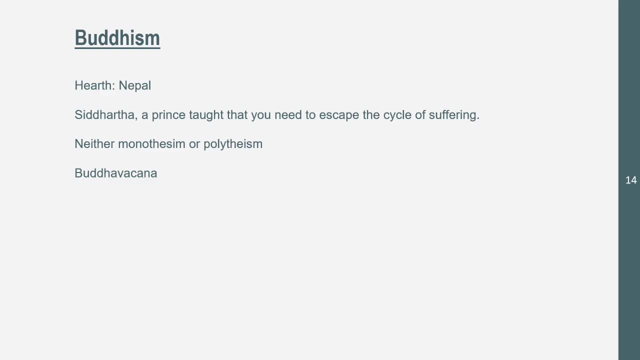 I'm not going to pronounce that, but you can read that on there. Now it's spread through contagious diffusion, through teachings, and then relocation diffusion, And this is very contemporary Buddhism is diffusing a lot, So there's a lot of relocation. 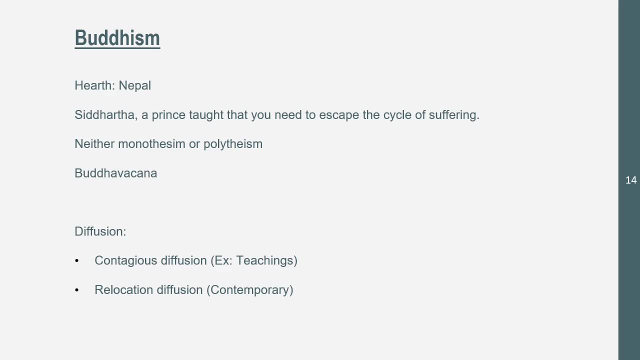 diffusion of Buddhism, And that's happening a lot now. Of course, it happened a lot back then, but it's really happening more now. Islam, The hearth is going to be in Saudi Arabia. Allah, which means God, shared information to the prophets who made Koran, which are the holy. 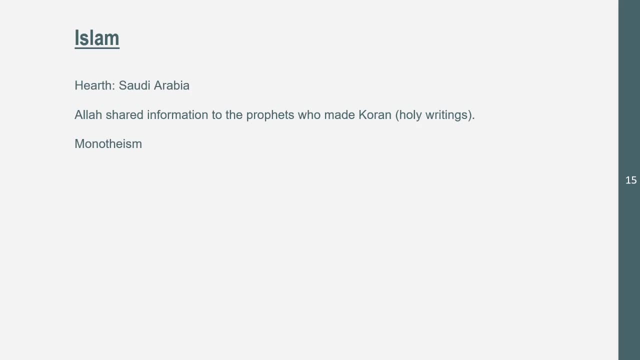 writings to the Islam. It is a monotheistic religion. They believe in Allah as the God And then their sacred text is Koran, And it's spread through contagious diffusion. Trade was a big part of spreading Islam And then relocation diffusion, especially from the Middle East to a bunch of Western 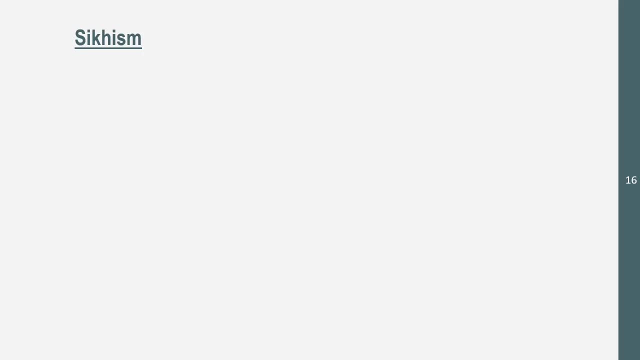 Asia and then Northern Africa. Now let's get into Sikhism, which is the hearth in Northern India under Nepal, though. One god is the creator of the universe and life is precious and should be So. it's a religion that should not be wasted. I hope I got some good summary. This is probably 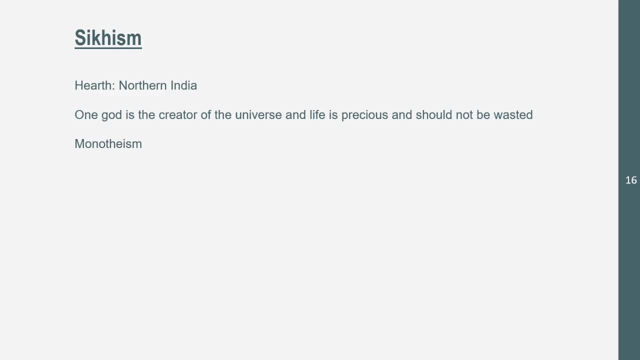 the worst summary out of all six religions. It is a monotheistic religion And its autograph is its sacred text, And it's spread through contagious diffusion, missionaries, and through relocation, diffusion, migration. Now let's get into our ethnic religions, which is religions appealing to one group. 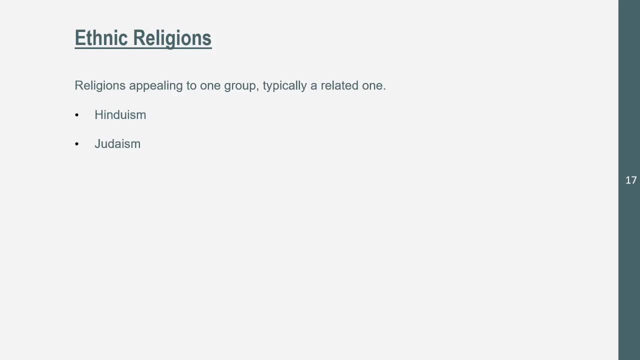 typically a related one. So we have Hinduism and Judaism as our ethnic religions. They're not going to diffuse as much as our universalizing religions, especially Christianity. All right, Hinduism is the hearth that's in Northern India, just like Sikhism. 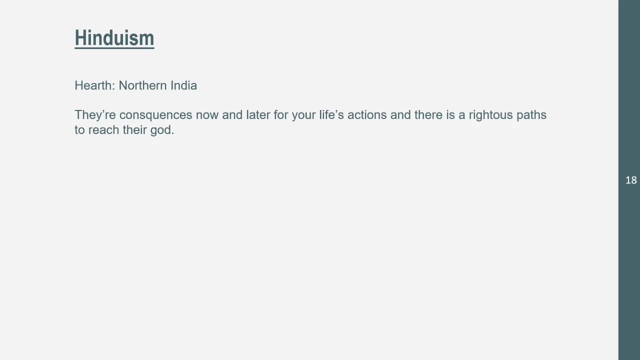 There are consequences, now and later, for your life's actions And there is a righteous path. There are righteous paths to reach their god or gods. It is polytheistic. They believe in multiple gods, millions of gods actually- And they are followed by the books of knowledge as their sacred texts. 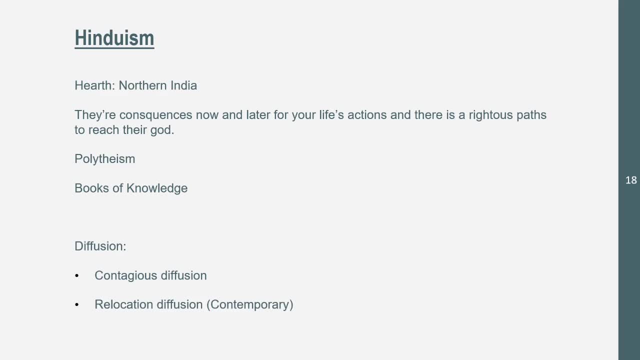 It's spread through contagious diffusion and through relocation diffusion. Relocation diffusion is more contemporary. I've seen a lot of migration patterns. I've seen a lot of migration patterns from India in the past. while I've been looking at past news articles for current events, for AP Human Geography and 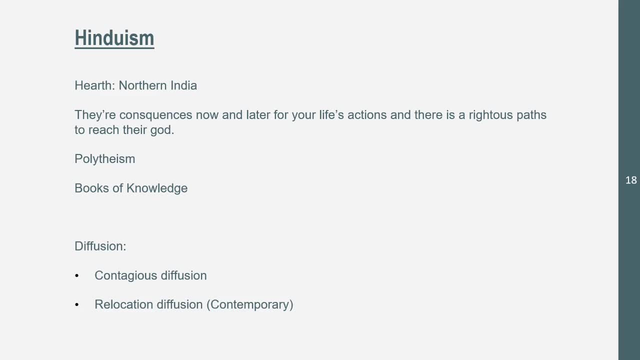 I've seen a lot of Hinduism diffusion, especially to America. Brain drain is pretty common there, from Unit 2, if you remember what brain drains were. Now let's get into Judaism. The hearth is in modern-day Israel. It was called, I believe, like Mecca or something. 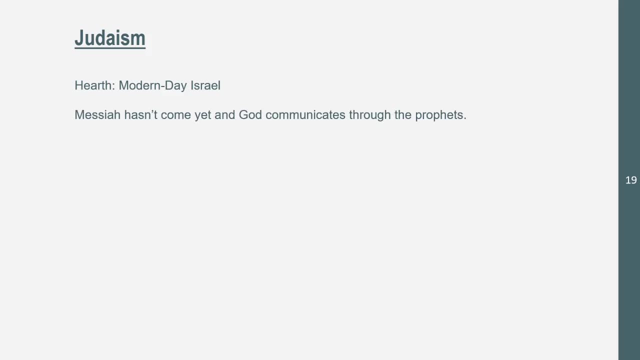 The Messiah hasn't come yet, and God communicates through the prophets. That's what they believe in, So they don't believe Jesus is the Messiah, Like Christians do. And then God communicates through the prophets And then someday there will be a Messiah. 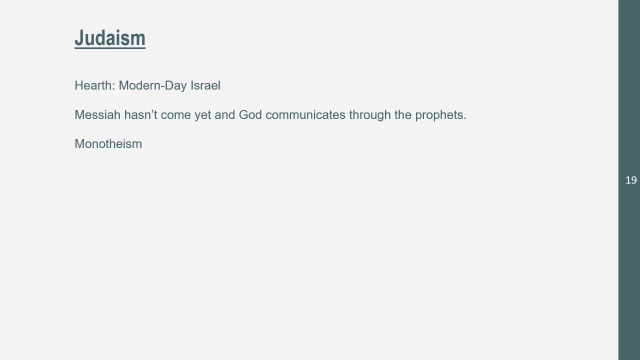 See how I use the word. yet It is a monotheistic religion. They believe in God, nothing else. And then their sacred text is the Tanaka- or Tanaki, Correct me somewhere- And it's spread through relocation diffusion. 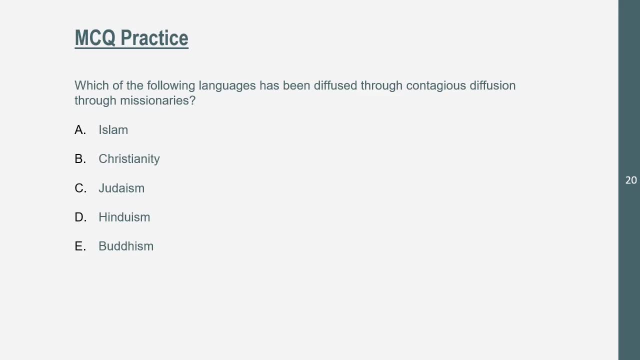 Now let's get to multiple-choice question practice. Which of the following languages has been diffused through contagious diffusion? through missionaries? So there may be some contagious diffusion here. What was it through missionaries? primarily? The correct answer is Christianity. Islam didn't spread for missionaries that much. 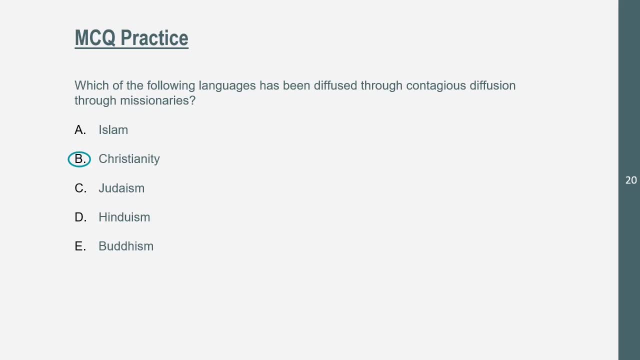 A lot of relocation diffusion. Judaism hasn't gone through contagious diffusion, Just relocation diffusion. And then Hinduism, Also an ethnic religion like Judaism, So it's not going to spread through much contagious diffusion. It did spread through contagious diffusion but not through primarily missionaries. 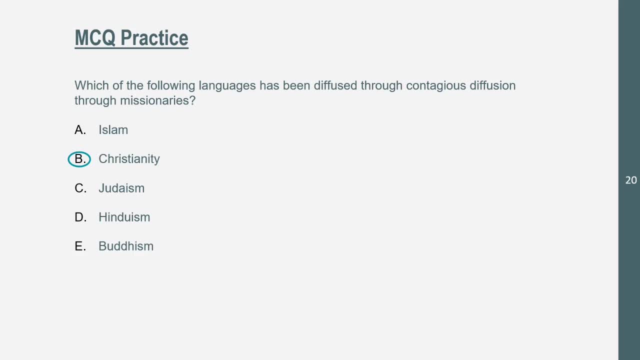 And then Buddhism was through a lot of teachings. when they did contagious diffusion- I wouldn't necessarily say missionaries would do that- This could be a tough question. You can probably see a question like this on your AP test. You might see something a little bit easier through a different type of diffusion.